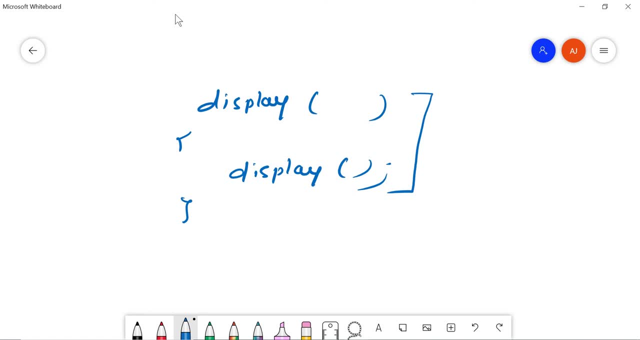 hope you understand the basic concept. Now let us explain or let us discuss about five differences for this: recursion and iteration. Okay, So I'll be writing here: First difference, So let us write iteration. and this is recursion. So first difference. Okay, So what is iteration? So the first. 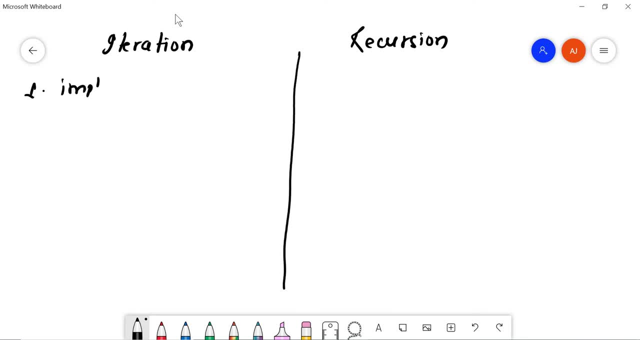 difference is iteration: It is implemented, Okay, It is implemented using loop. And in recursion it is implemented, Okay, Implemented using loop, Function, call, Function, call, Right. So next it is, if you see difference number two, Okay, So in. 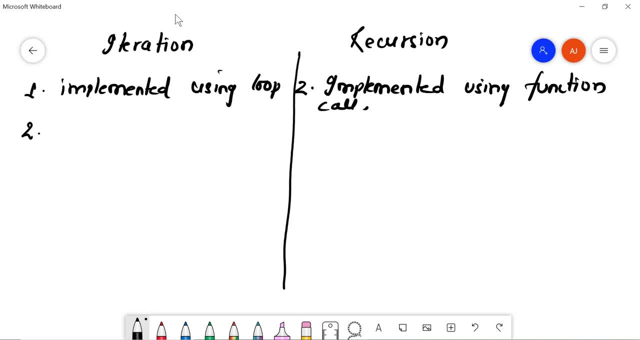 iteration. what happens is it is terminated Okay When the condition fails, For example in loop. when it is terminated, so termination occurs. Termination occurs when the loop- let us say condition- fails Okay. So, for example, when i in the previous case, 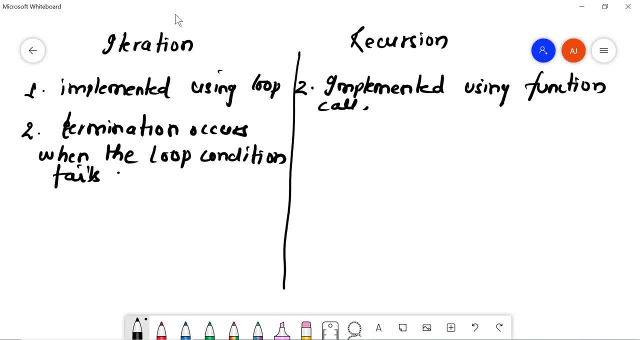 if value of i becomes equal to 10.. So 10 is less than equals to 10.. It is false, So it terminates. The loop terminates And in case of sorry, this is one number In case of recursion. Okay, So it is. 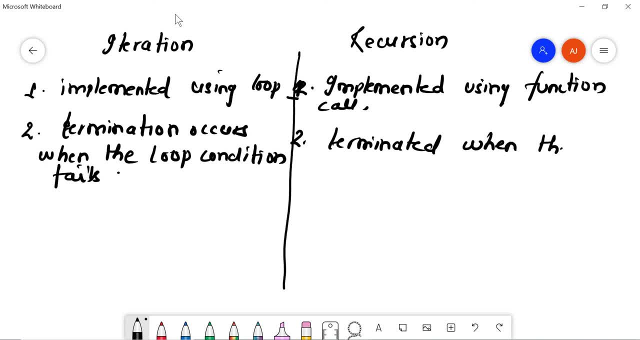 terminated when the base condition is fulfilled. Okay, So remember, recursion, recursion, recursion in function or recursive function. we have, we always have a base condition. So when the base condition is completed, the recursion gets completed. So in this way, this is for recursion. Okay, Next is: 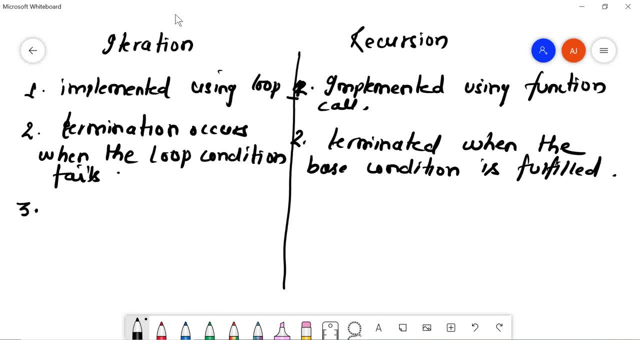 in number three, we can write: okay, So, when this infinite condition occurs. Okay, So, infinite loop. you have heard about infinite loop. Okay, So when this infinite loop occurs, so it infinite loop is there. Okay, Infinite loop is there if condition never fails. 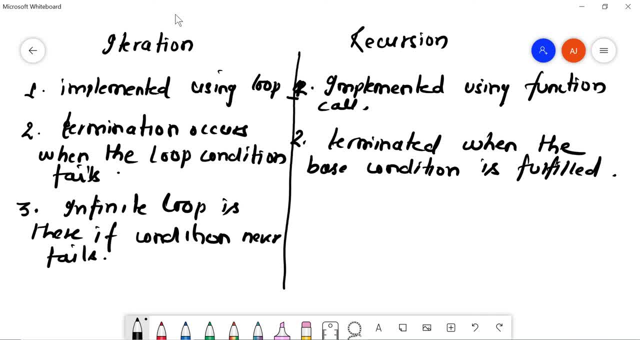 Okay If you will put a condition that will never fail. So in this case, infinite loop occurs, Fine. And in case of recursion, infinite recursion occurs. Infinite recursion occurs, Okay, If there is no base condition, if there is no base condition. So if you remember the 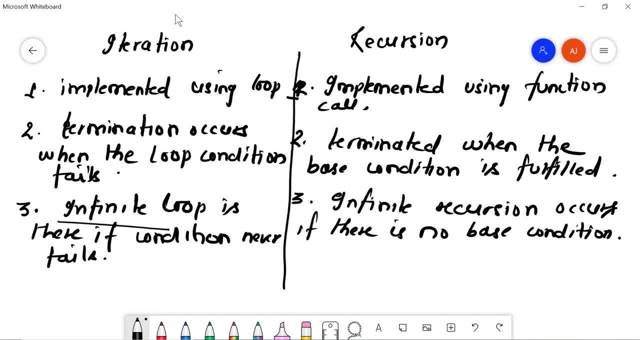 properties of recursion. so this is one of the mandatory case that you must have. Okay, You must have a base condition, Fine. So next difference we can say is: it runs slower. Okay, It is slower in case of processor also, And it runs faster. 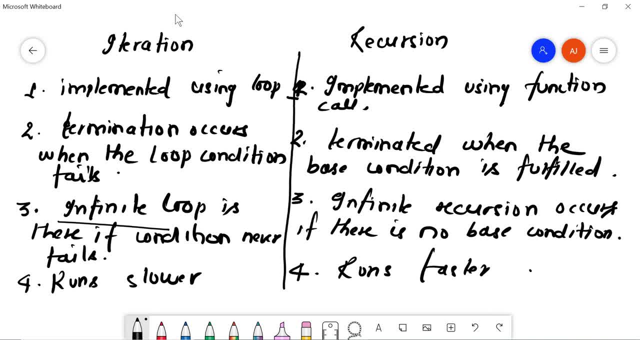 It is faster than iteration: Fine. So these are four differences: Fine. And another difference: you can write here like: it requires it requires more storage, Fine. And pipe number: you can write: it requires less storage. So I think this is more than enough, And one difference you can. 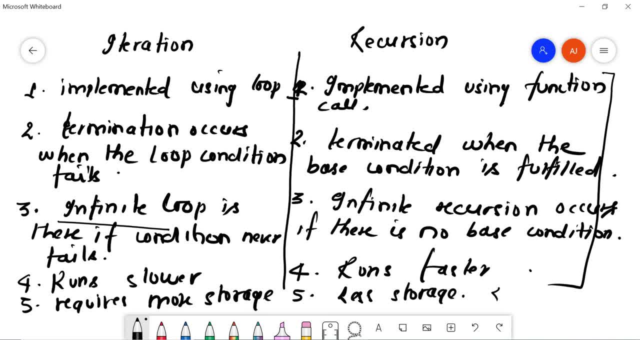 give the example, as I have done in the starting of the video, So you can give one example for this. So I think this is more than enough And this is one of the important question. Okay, So this can be asked for four marks to five marks. Fine, Sorry for the. 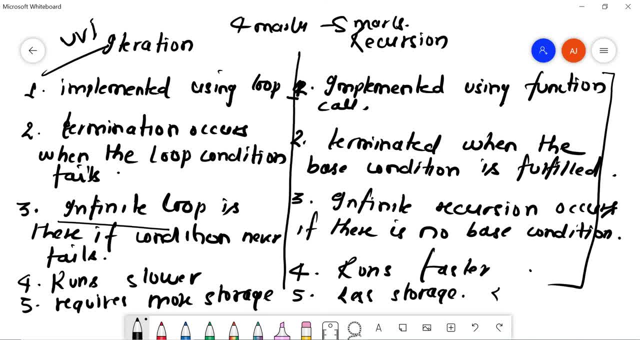 writing And hope you understand this video, So next I will be coming with another question discussion. Thank you and stay safe.